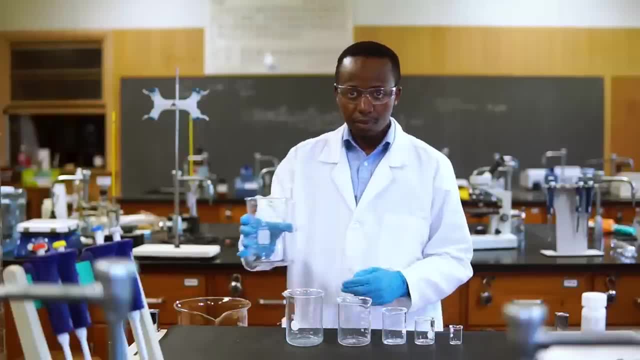 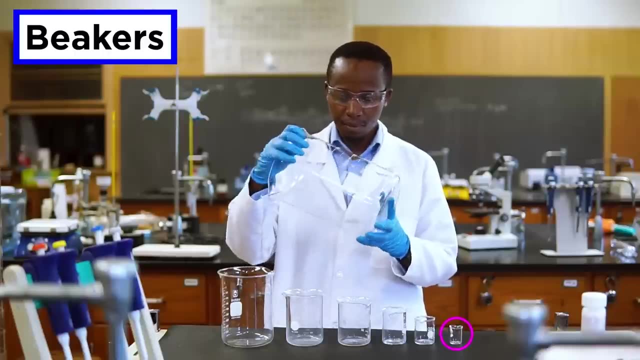 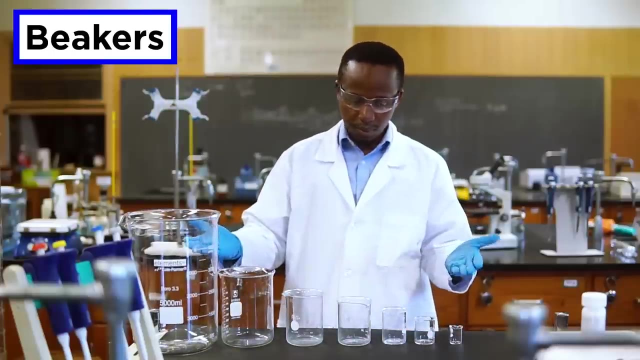 lots of glassware. Let's start with one of the more familiar items. These are beakers. There is a range of beaker sizes available, ranging from as small as 5 milliliters to as large as several liters, and there are different situations in which these different sizes would be desirable. 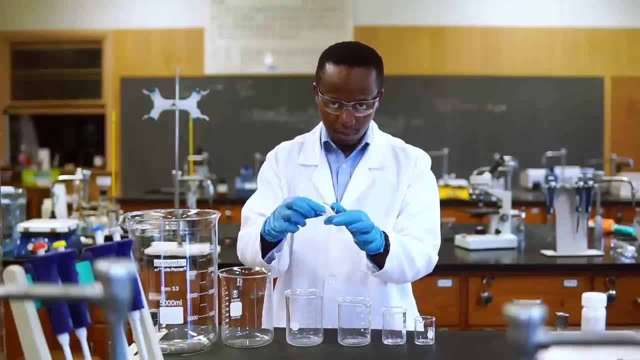 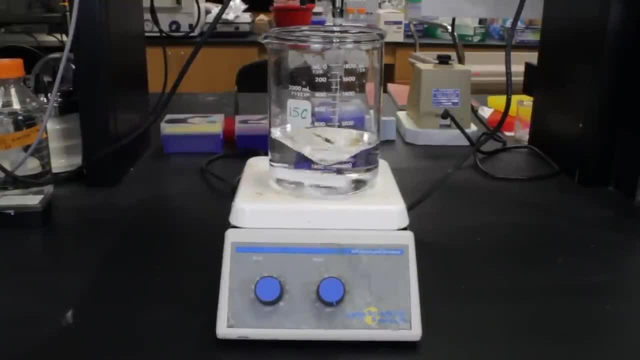 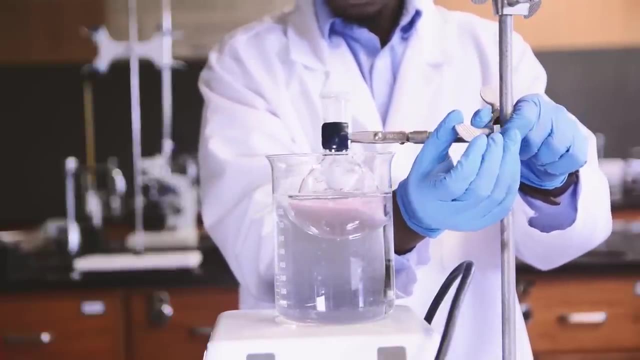 Most often, we tend to use beakers between around 10 to 400 milliliters. Beakers have many uses. Reactions can be conducted in them, They can be used to transport solutions and solvents, Or they can be used as water baths, meaning we can suspend some other vessel in the 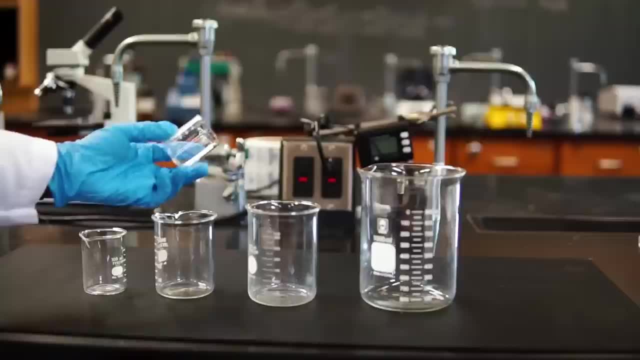 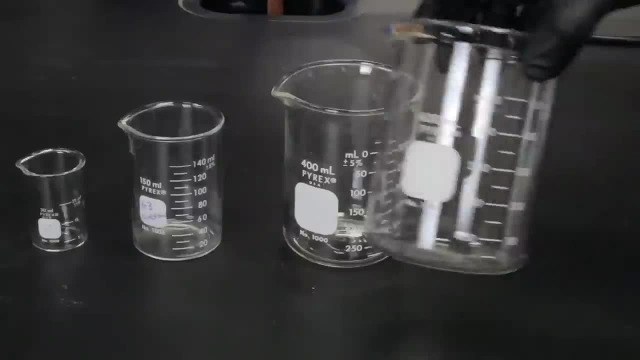 beaker in order to control its temperature. Always be aware of what you are using a beaker for and use the appropriately sized beaker for the job. The measurements on the side of the beaker are great for estimating the volume, but we do not carry out actual measurements of volume using 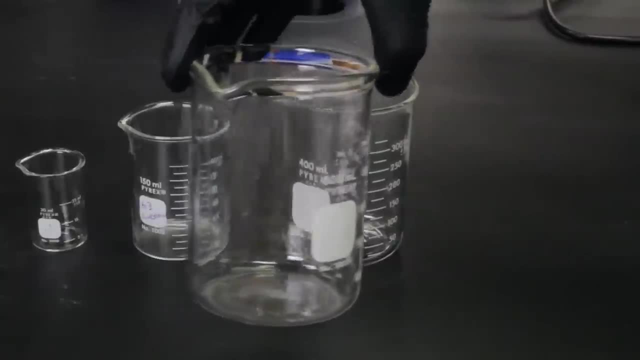 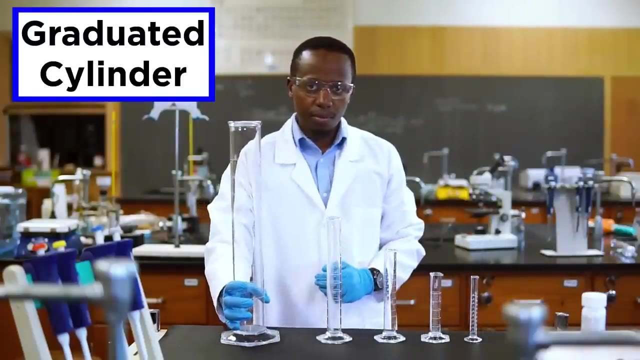 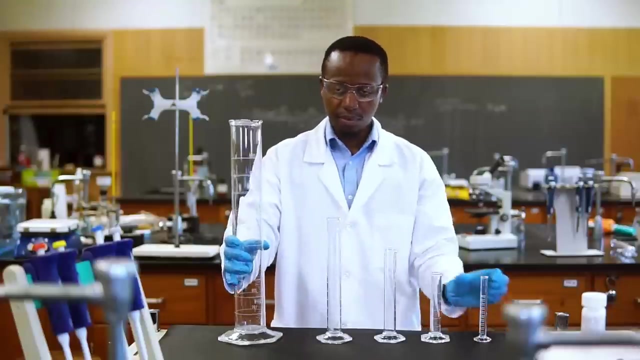 beakers. We have glassware that is more accurate for measuring volumes when necessary. Speaking of measuring volumes, next up we have the graduated cylinder. A graduated cylinder is used to measure the volume of a liquid. These also range quite a bit in size. Be aware that they are tall, so you. 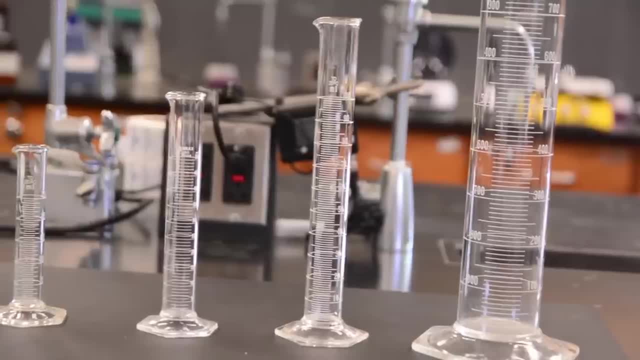 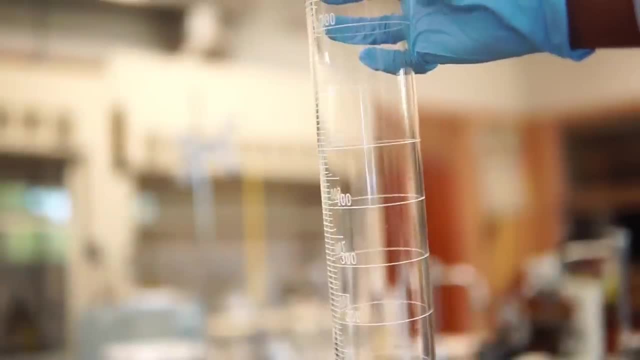 may at some point accidentally knock one over. In order to avoid this, always place them down where you can see them or where less movement is occurring. We should also be aware that when taking measurements with a graduated cylinder, we will always read from the bottom of this concave. 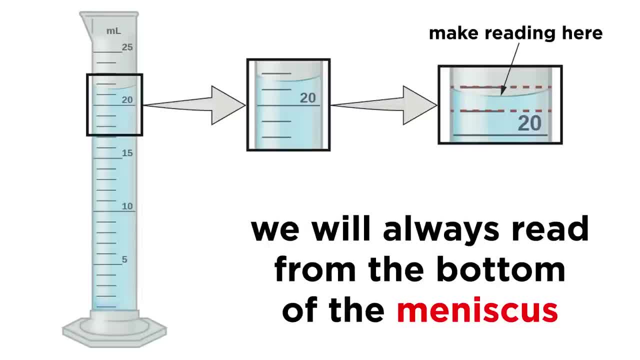 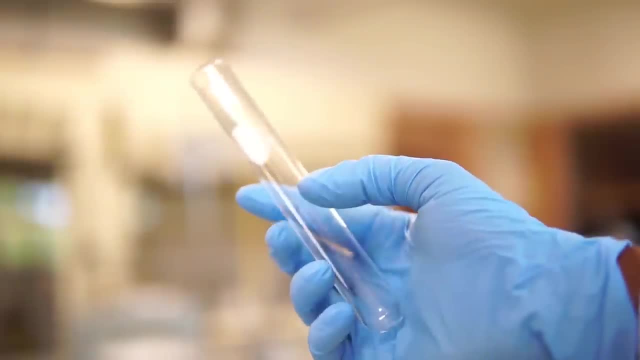 meniscus. This word refers to the way the liquid climbs a little bit up the edges, and to avoid ambiguity, we will take readings from this position here. Next we have test tubes, test tube racks and test tube holders. A test tube is a very small reaction vessel. 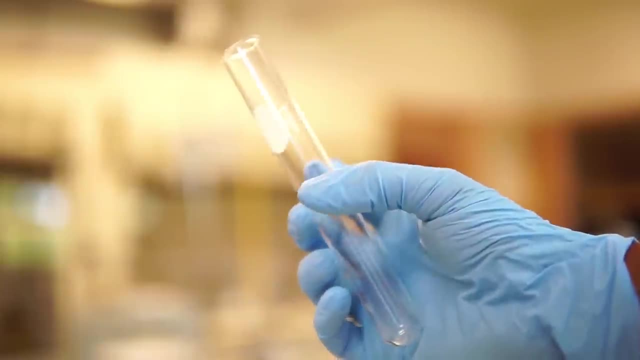 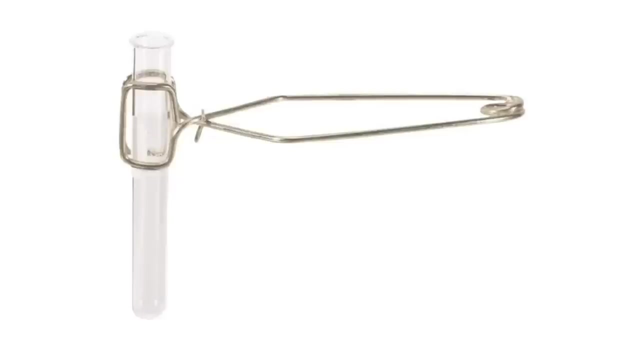 which is nice to use when observing obvious, visible changes in the reaction. They don't stand up by themselves, so be sure to place them in a test tube rack so they don't roll away. A test tube holder like this one can be used to hold a test tube above the flame of a Bunsen burner. 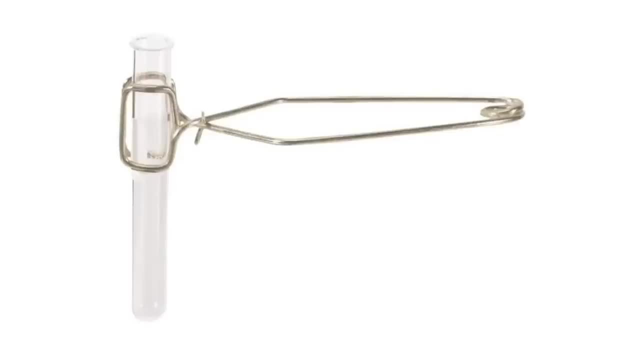 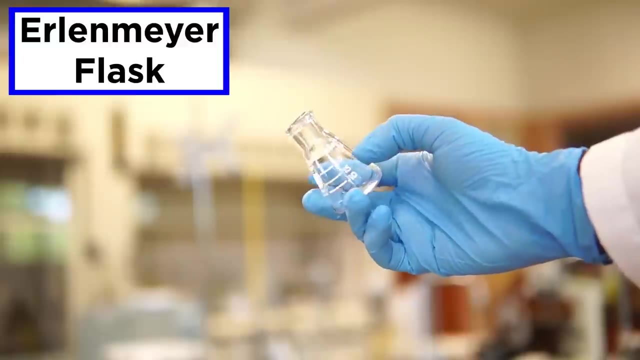 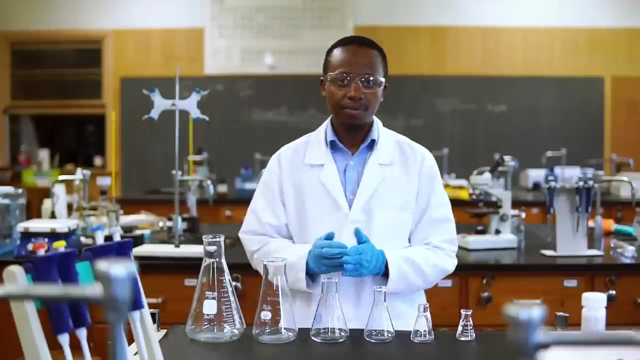 or suspend it in a water bath. Get comfortable holding one of these before heating it, and be sure to have one that fits the size of the test tube you are using. Next, let's check out another recognizable piece of glassware: The Erlenmeyer flask. A conical or Erlenmeyer flask looks like this. These are typically used. 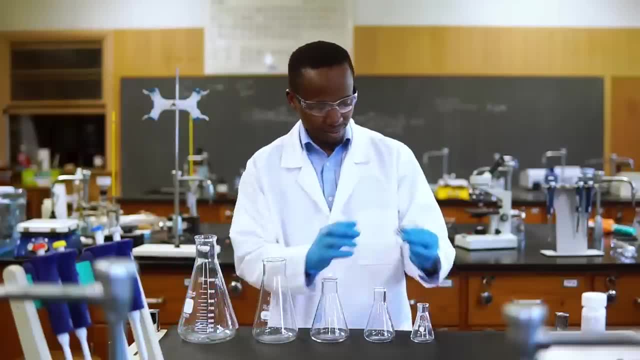 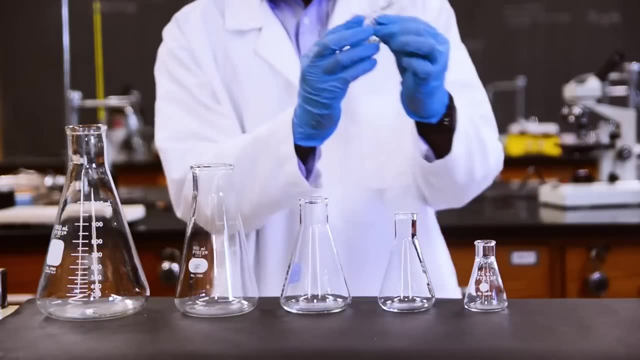 for mixing reagents together and conducting a reaction. Again, they come in various sizes and the measurements on the sides are quite imprecise, so they shouldn't be used when accuracy is necessary. The tapered edges leading to the small opening at the top prevent spilling. 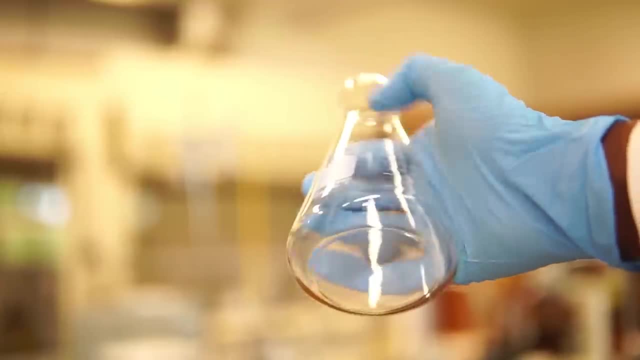 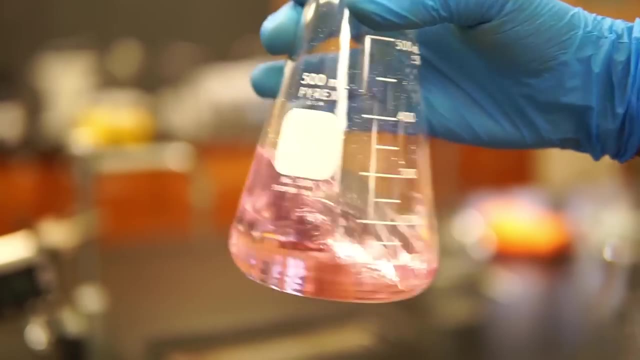 and they also make these flasks ideal for clamping, which is something we will commonly want to do. If the mixture needs to be manually stirred, you can manipulate them with less fear of the solution escaping, which is why these are typically preferred for running reactions over beakers. 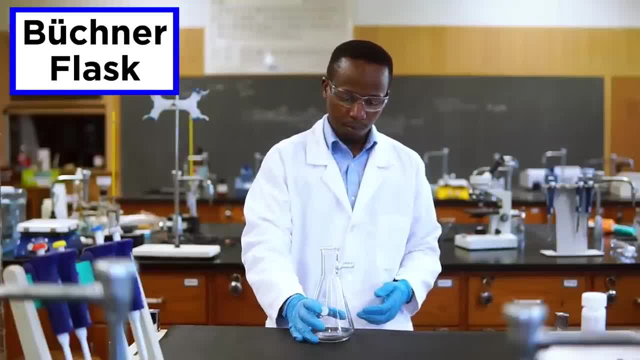 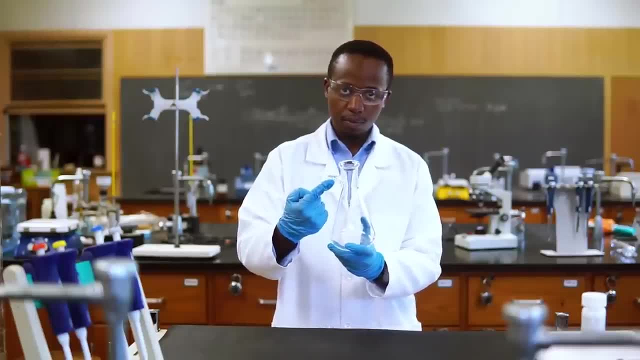 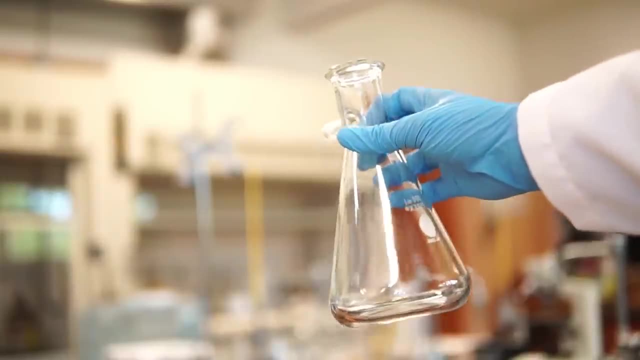 Next, we have the indispensable Buchner flask or filter flask. These are very similar to the Erlenmeyer flask. it is simply that the Buchner flask has a side arm which is used when conducting vacuum filtration, which we will discuss in another tutorial. Avoid using these for anything. 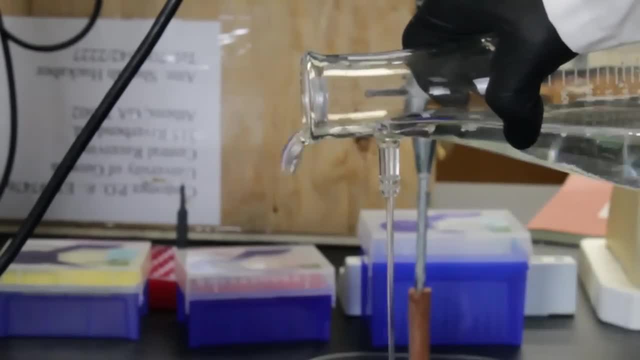 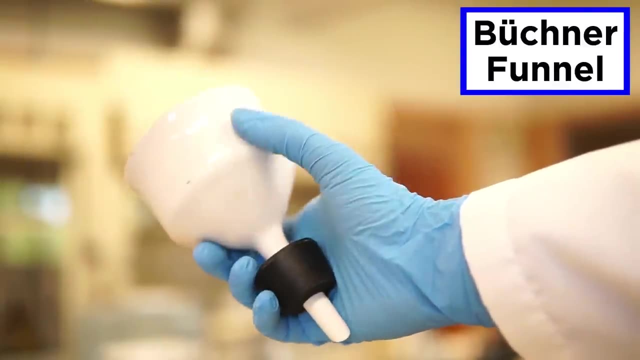 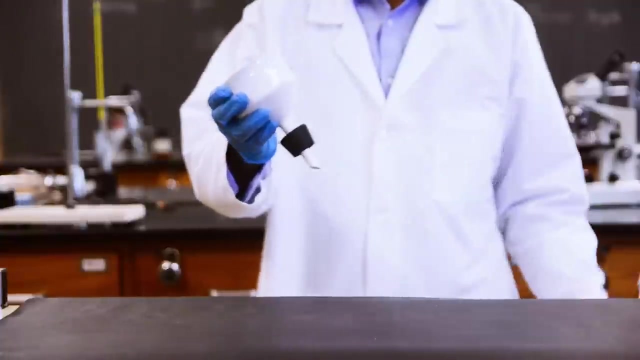 else, as the side arm opening can cause the liquid to escape. With the Buchner flask covered, let's check out the Buchner funnel and accompanying rubber adapter. The Buchner funnel is also used when conducting vacuum filtrations. These sit in the Buchner flask. 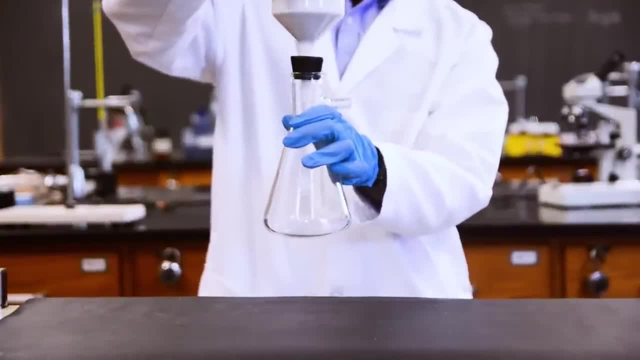 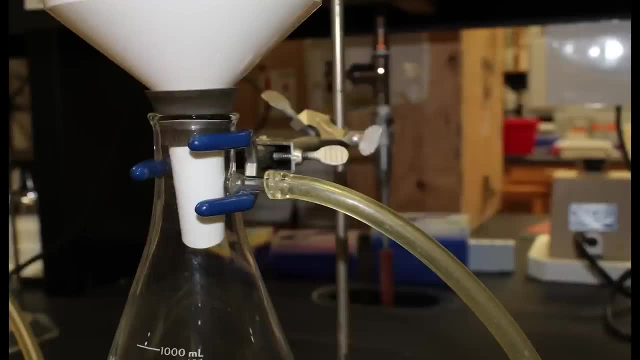 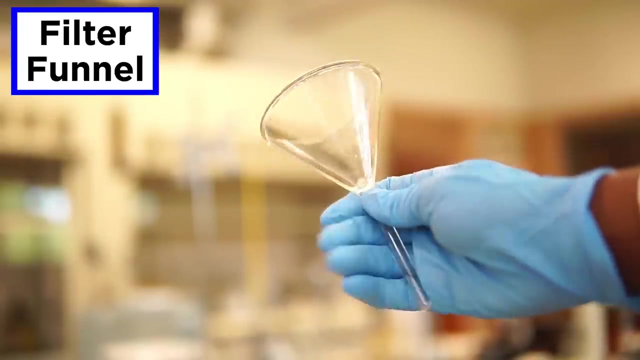 and are typically made of ceramic, but plastic ones are sometimes used. For a better seal, we tend to use the rubber adapter. These aren't all that stable, so be sure to clamp the flask first before assembling the filtration setup. Next let's examine the filter funnel. For gravity filtrations we use this kind of funnel. 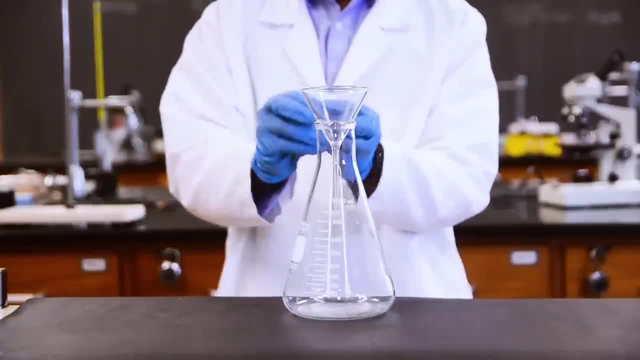 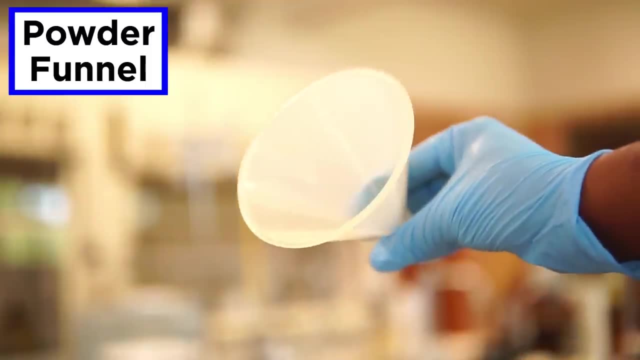 Either cotton wool or a folded piece of filter paper can be used for gravity filtrations, which will also be properly demonstrated later. To finish off the funnels, let's check out the powder funnel When wanting to add powder to a flask, which could be a drying agent or any. 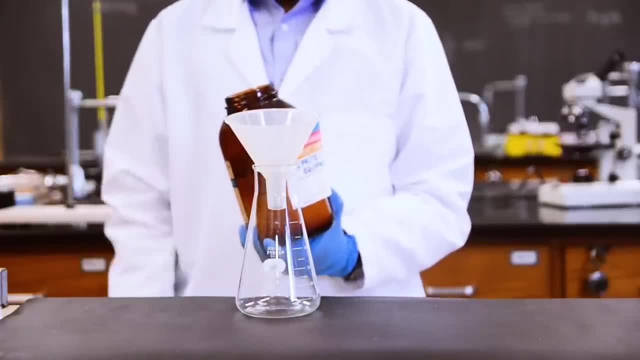 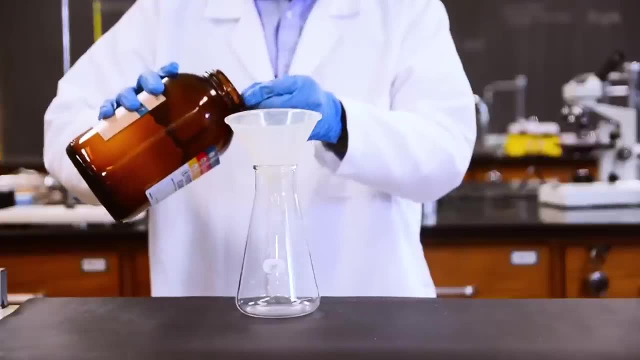 solid reagent. sometimes it is necessary to add a little bit of powder to the flask. If you want to add powder to a flask, it is much easier to use a powder funnel. These can be placed on top of a flask and a solid can be added easily. These typically are not made of glass, so they are easily. 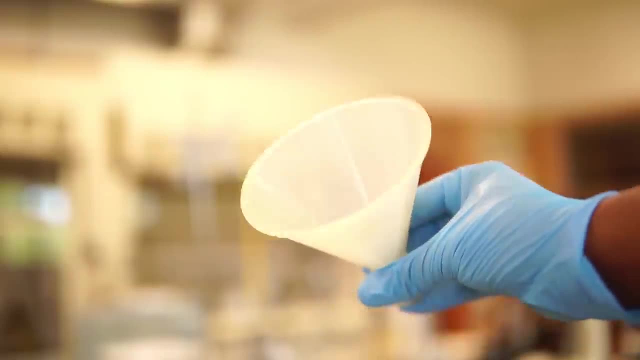 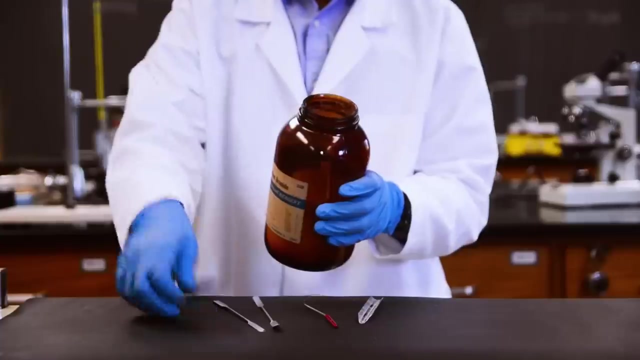 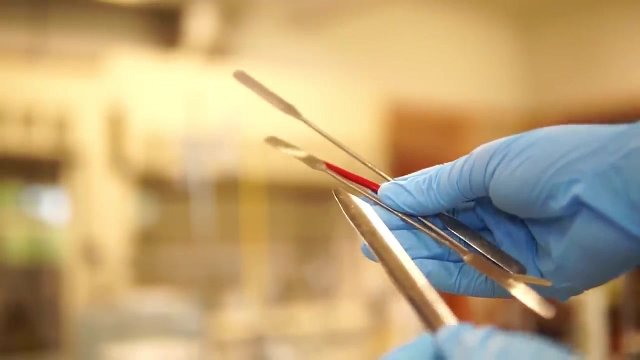 distinguishable from the other funnels. Be sure to check and see if it is clean before using it and clean it afterwards. Next, we have the spatula. When picking up solids, we will use a spatula. Some are curved, some are flat, and they usually bend if necessary, but be gentle whenever possible. 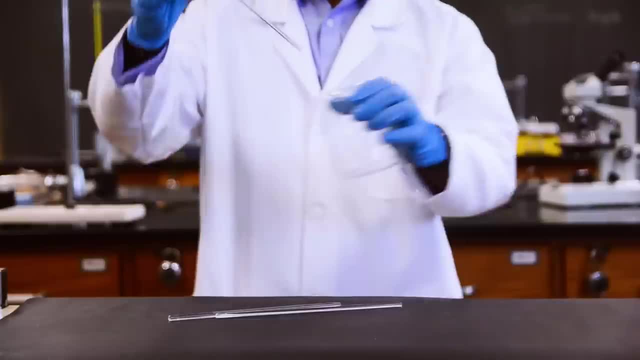 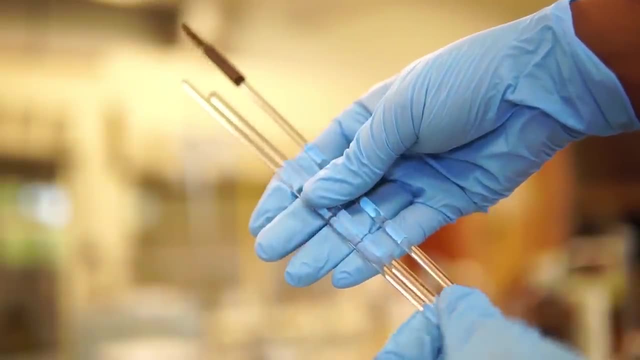 Similarly, we have the stirring rod. When wanting to briefly stir something, a stirring rod is the best option. Do not get this confused with a thermometer and be careful when putting these down, as they do roll away. Then we get to the pipette For adding small amounts of liquid. 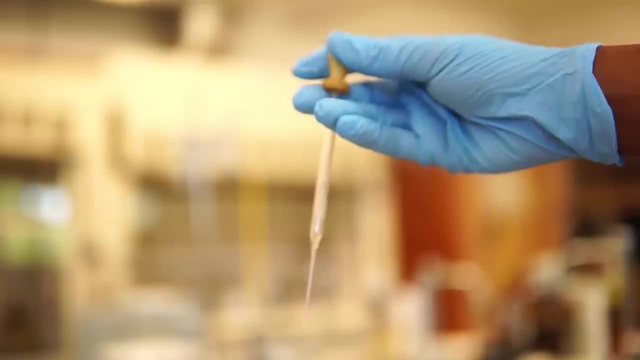 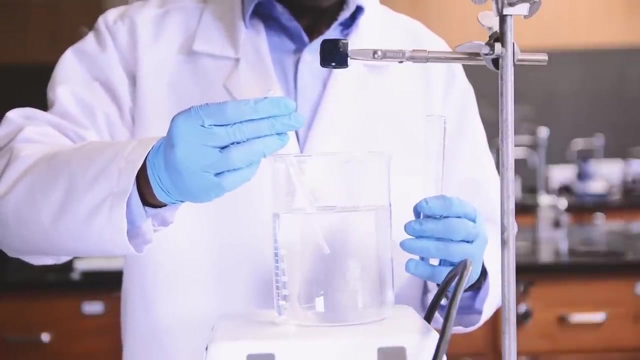 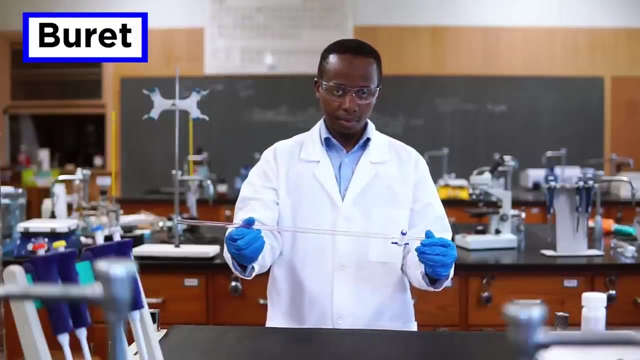 we use a pipette. Using a pipette bulb, a liquid can be taken up and put somewhere else. Simply squeeze, place into the liquid, release the bulb to draw the liquid into the pipette and then transfer it to the new vessel Next up we have the burette. These are commonly used. 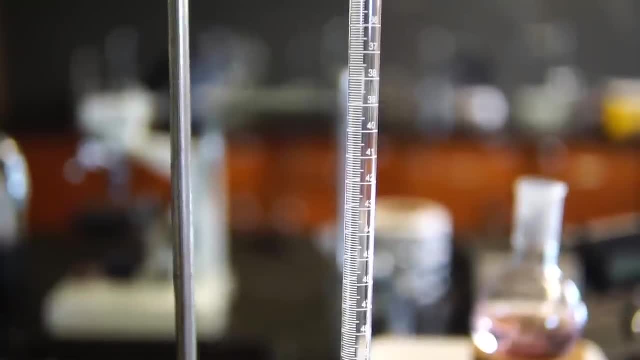 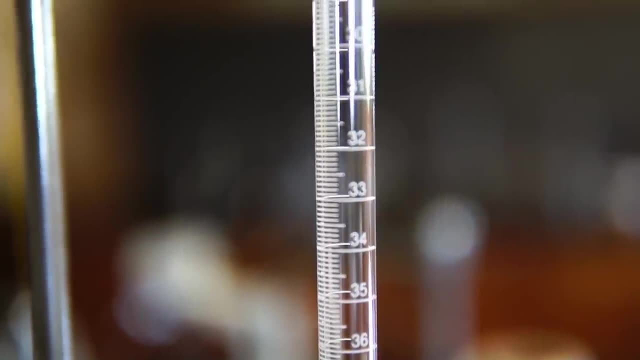 with titrations, Like a graduated cylinder. it has these gradations for measuring volume, but unlike a graduated cylinder they are inverted so that you can measure how much volume is being added to some other vessel. A more thorough demonstration of this instrument will be shown. 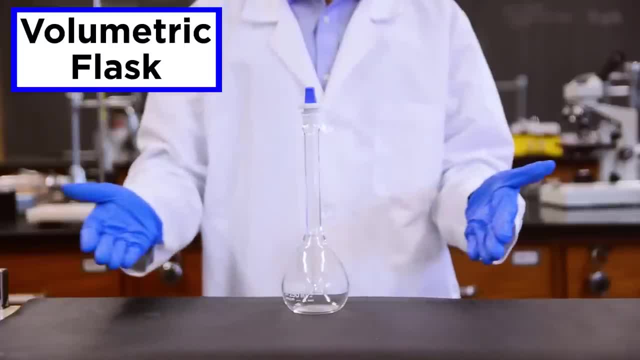 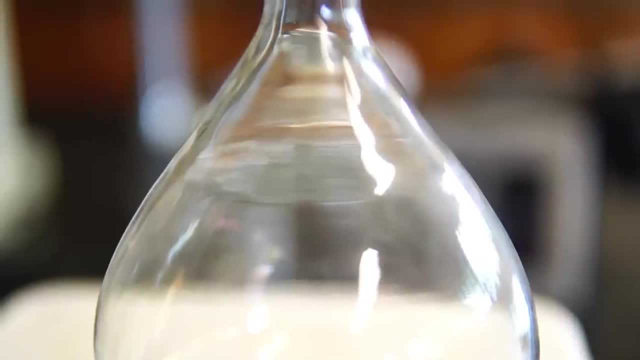 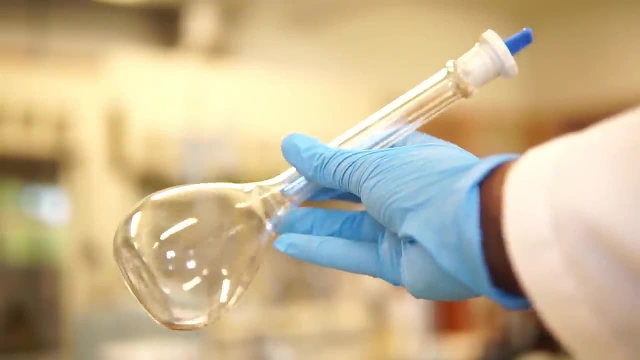 when we conduct a titration. Then there is the volumetric flask. When making standard solutions, we use a volumetric flask, Much like the volumetric pipette. a single line indicates the exact volume of this flask. Because of the long necks, these can be knocked over. 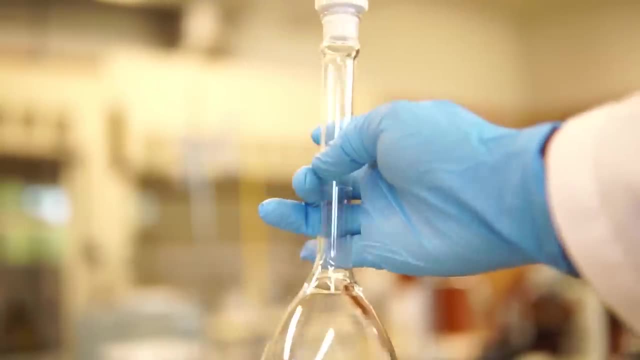 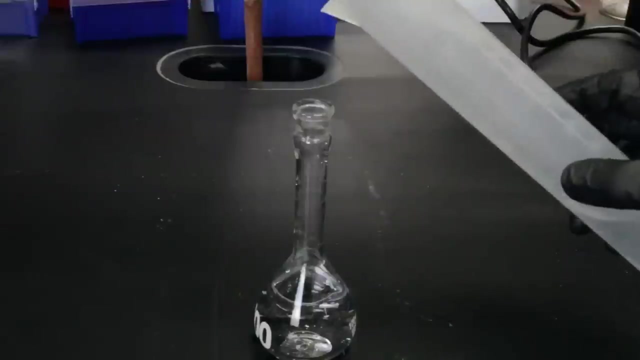 so, like the graduated cylinders, be careful where you place them. Also, check which cap you have, as some fit nicely, but others are deceptive. When using these to make solutions, be extra careful once you reach the neck, as this will fill up much more rapidly than the bulb, as it is so narrow. 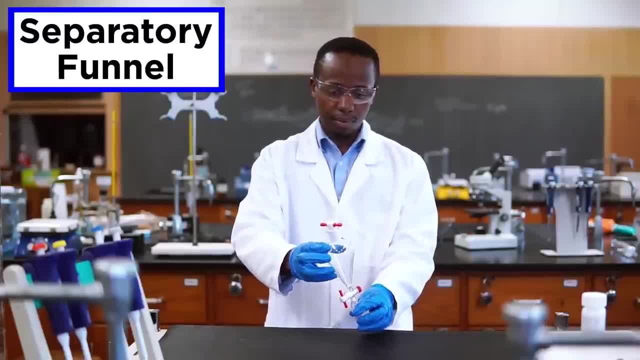 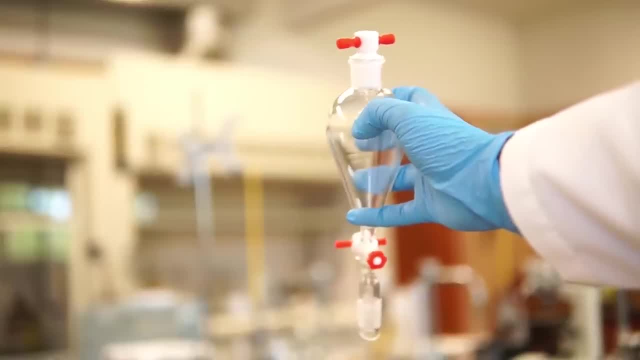 Moving along, we find the separatory funnel, which we learned about when going over extraction in the organic chemistry series, For separating two immiscible liquids. we will use a separatory funnel, sometimes abbreviated as a sep funnel. When using these, make sure you have the correct 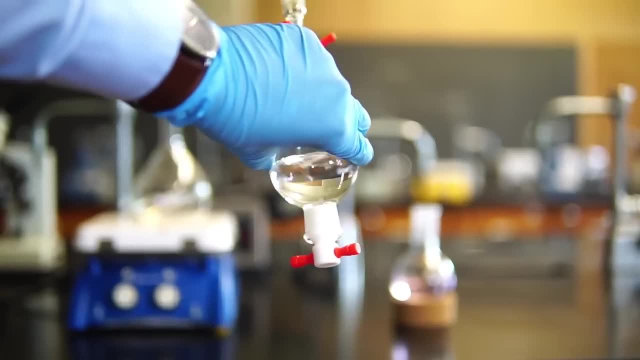 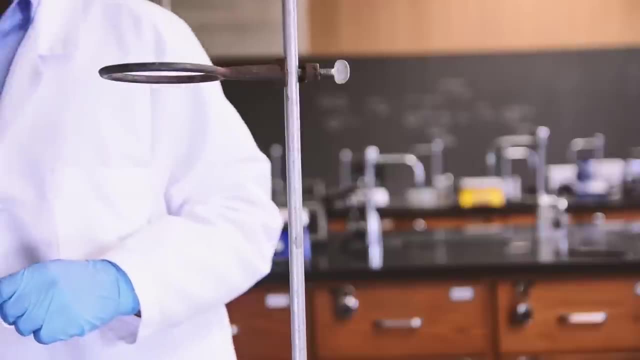 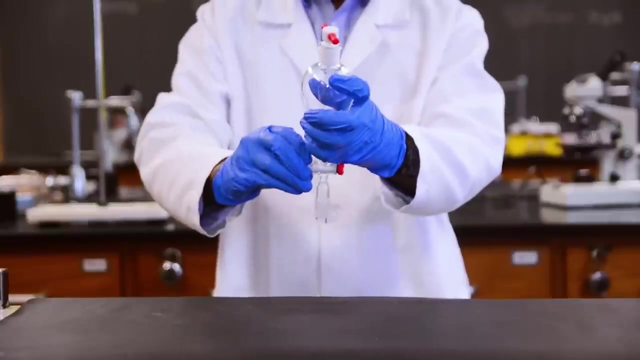 size cap so that nothing spills when inverted. Sep funnels require a ring clamp, so make sure that the size of your ring clamp is appropriate, as if too small the funnel will be unstable, but if too big it will not hold the funnel at all. We will notice that the separatory 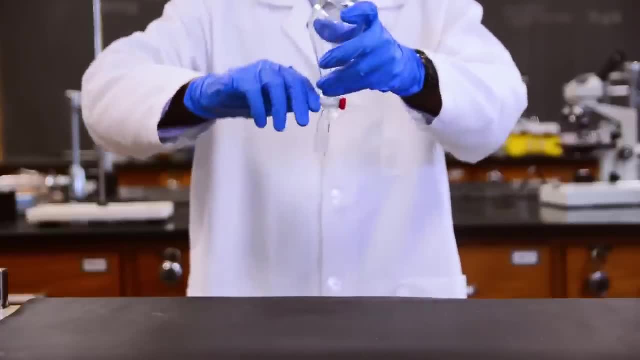 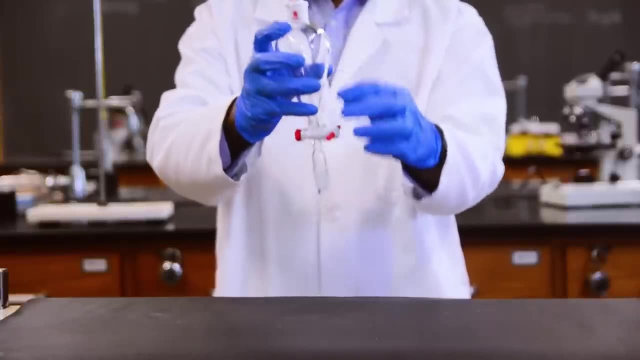 funnel has a valve for releasing liquid. Sometimes the valve comes assembled and sometimes they need to be assembled. We will talk more about this apparatus when we perform an extraction. Now this is called a dropping funnel. A dropping funnel looks very similar to a sep funnel. 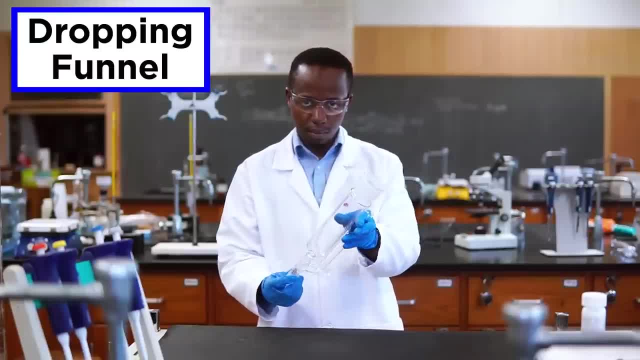 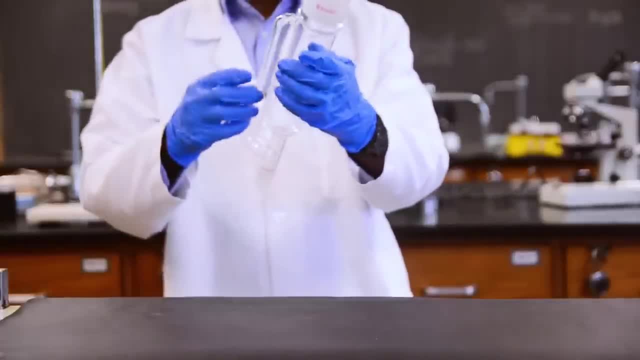 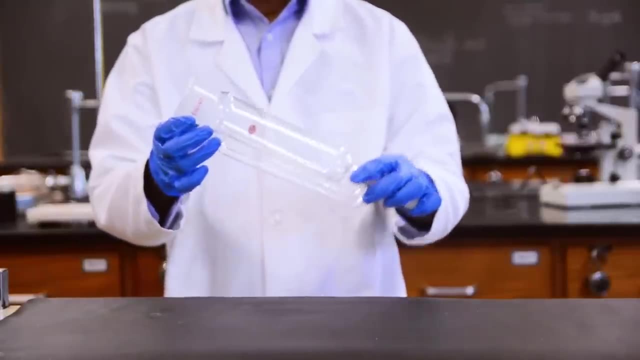 but they have this separate arm and a ground glass joint. These joints become important when you are doing reactions under nitrogen or argon atmosphere with air sensitive reagents and products. They are used to control the addition of a liquid to a reaction and the arm keeps the 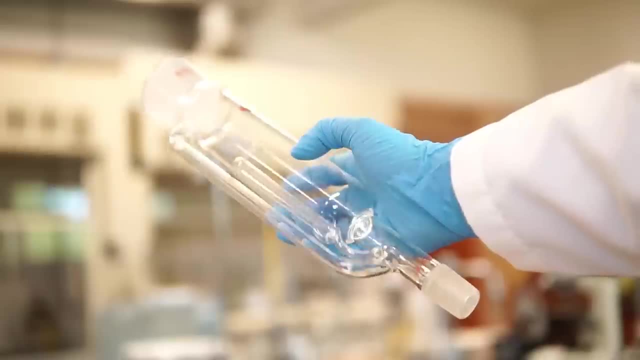 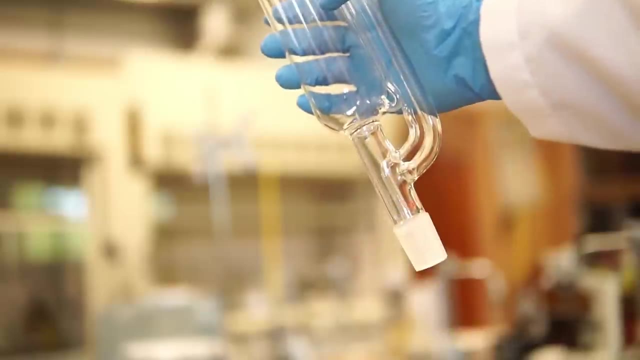 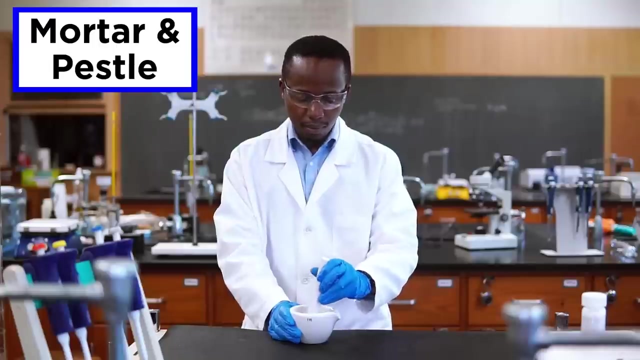 pressure constant, so the addition is smooth and continuous. If there is no need for the ground glass joint, a sep funnel will often suffice as a dropping funnel, but it is good to know what this is if you come across one. Next we find the mortar and pestle. If you need to crush up some solid 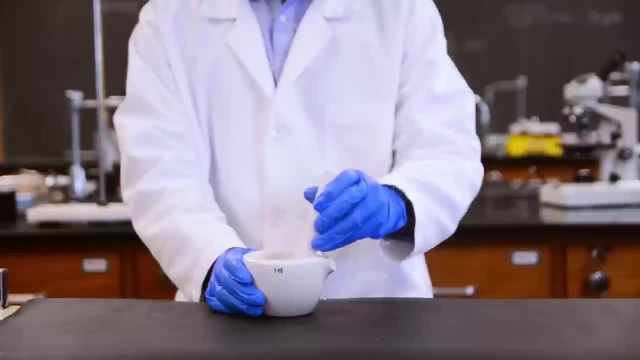 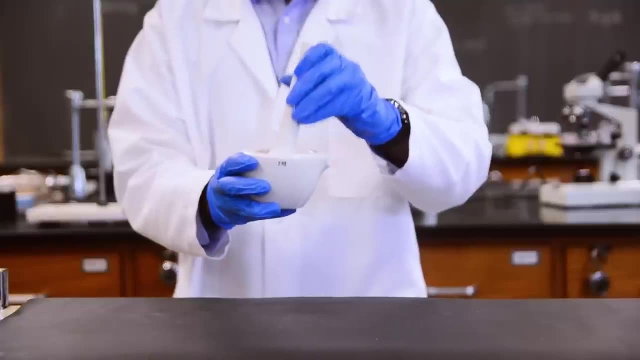 material into a powder, use a sep funnel. If you need to crush up some solid material into a powder, you'd use a mortar and pestle. These are pretty simple: you simply put the material in the mortar and crush it with the pestle. These are usually ceramic and quite heavy, and they are fun to use. 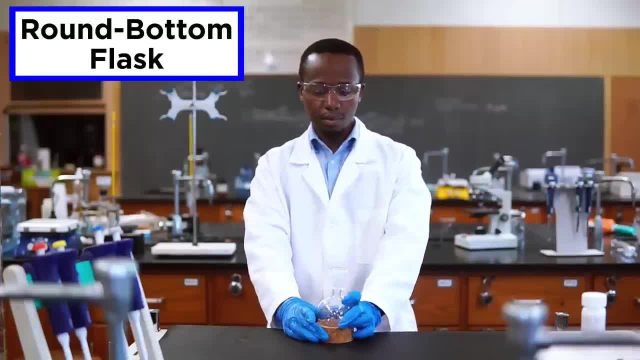 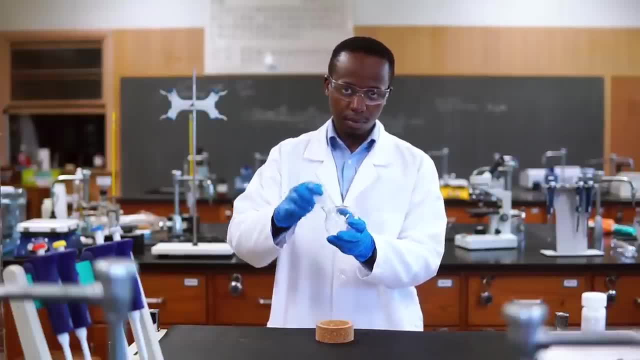 Now we get to that ubiquitous piece of glassware for the organic chemist: the round bottom flask. As we will come to see, for more serious reactions we will use a round bottom flask. There are many sizes and they almost always have at least one ground glass joint in them. 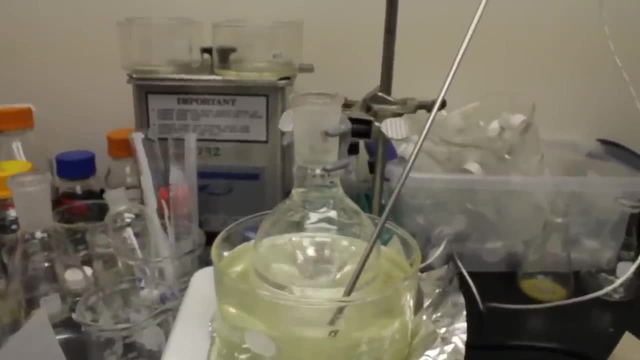 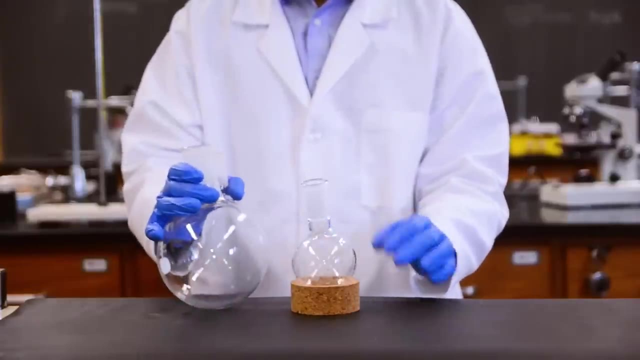 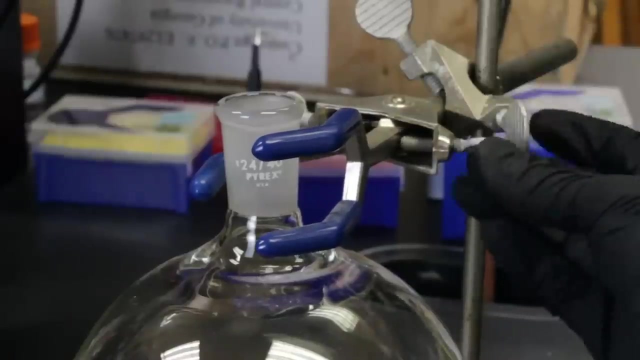 The roundness allows for better heat distribution and stirring where the joints allow for easy fitting with other glassware. Since they don't stand on their own, we will use a cork ring to hold them up, which must be of an appropriate size If securing to a solid support be sure. 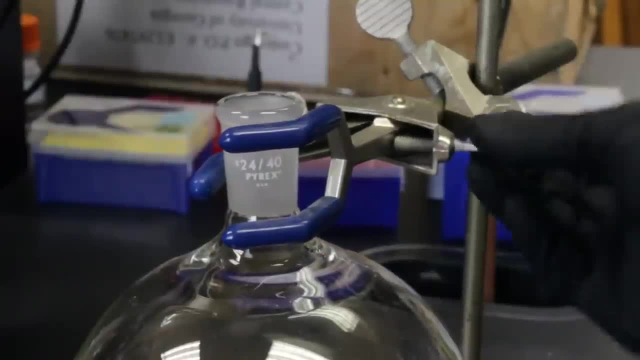 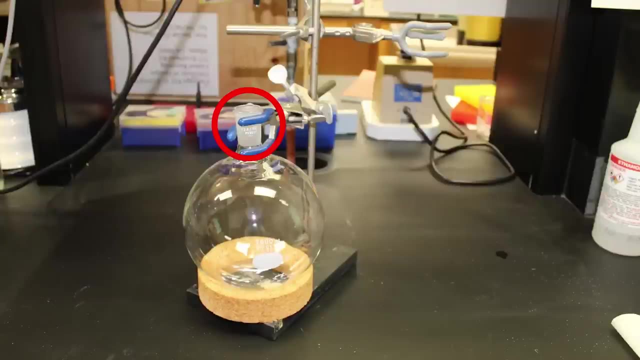 to clamp them around the ground glass joint area, as this is where the glass is the toughest. To be clear, this goes for all glassware. the ground glass joint is the thickest part and should be the area clamped by the joint For the round bottom flask. we have to clamp it on the 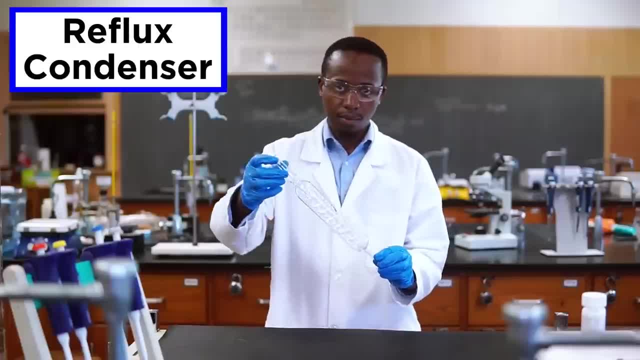 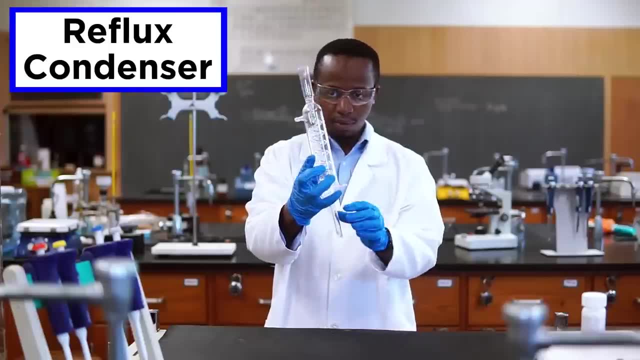 clamped whenever possible, Moving along. this is a reflux condenser. When we want to boil a liquid but don't want to lose any of the volume, we will use a reflux condenser. These can look very different from one another, but they are all used the same way. 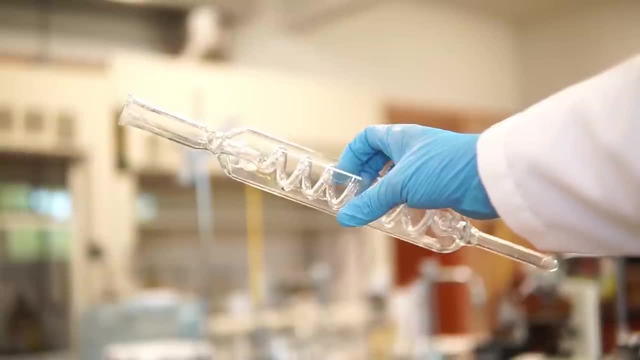 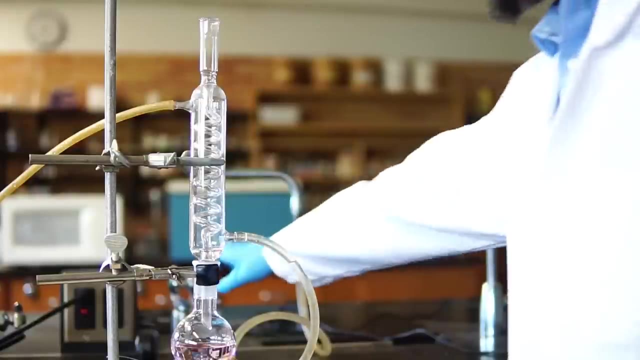 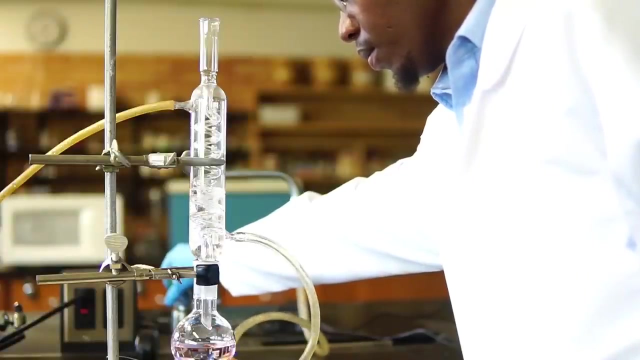 They are essentially a tube with a jacket, although some are just a tube, but these are less reliable. The glass jacket is filled with water through these side arms, which cools the environment in the tube, allowing for the gas to condense and drip back into the solution. 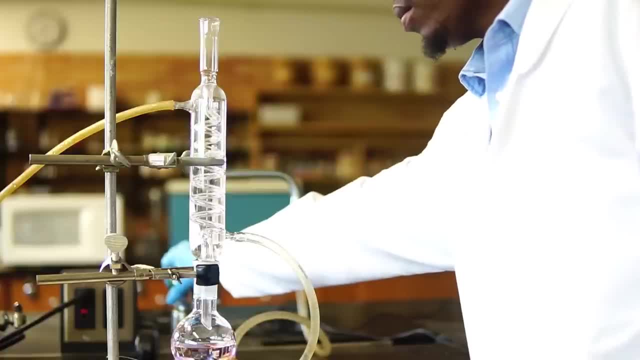 In this way, the liquid is always boiling but never escapes the reaction vessel. Tubes are attached to the arms here, with water flowing in from the bottom and out the top through a separate tube. It is very important to mention that we must never block the top of the condenser with 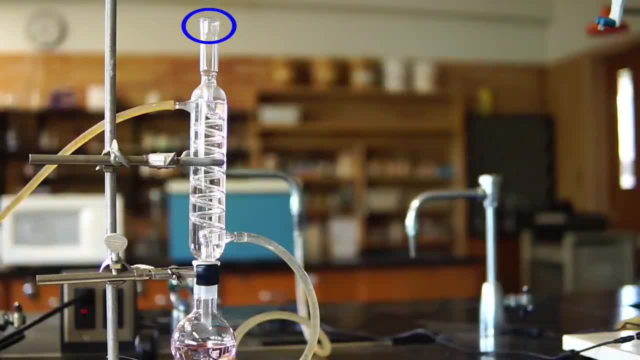 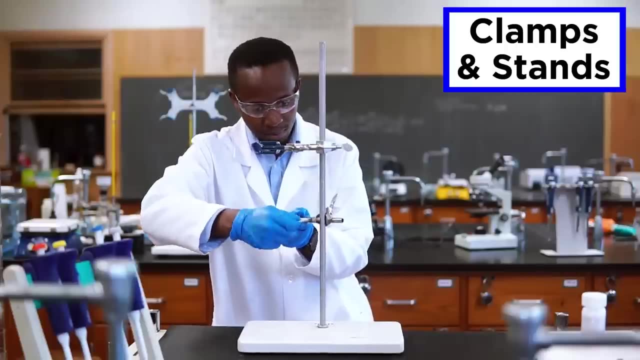 anything, as this will cause the pressure to build up, which could result in an accident. A more thorough demonstration of this apparatus will be conducted later. Here we have some clamps and a clamp stand, something we've already seen a few times by now. 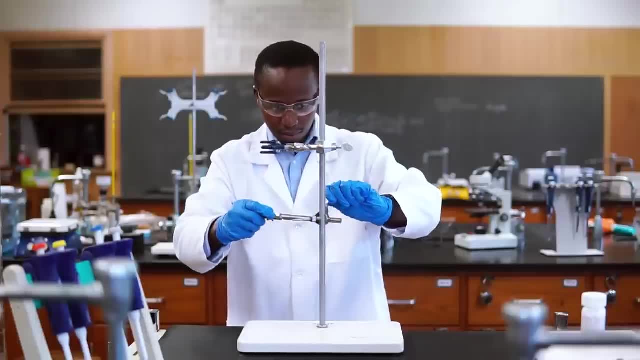 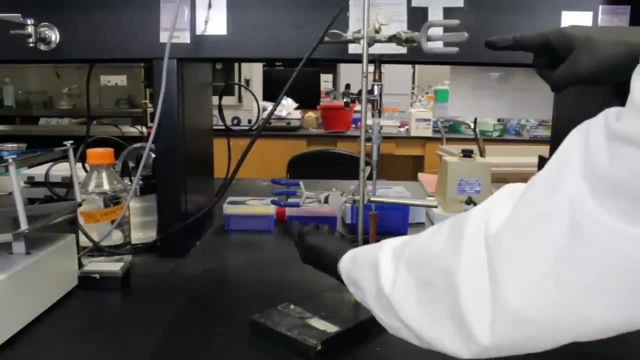 As you have likely gathered, these are used to hold up glassware and keep them locked in place. When using these, be careful with the weight distribution, as we don't want the clamp stand to topple over. The base may jut out in one direction more than another, so don't overload one side. 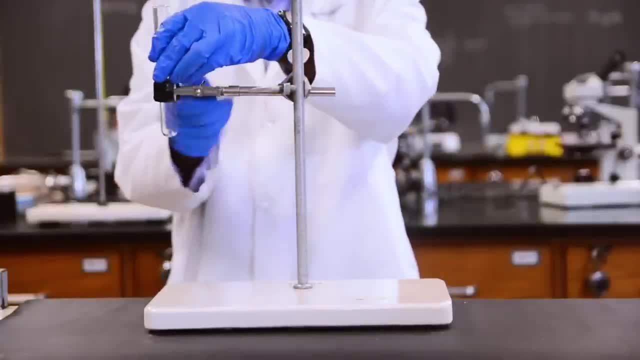 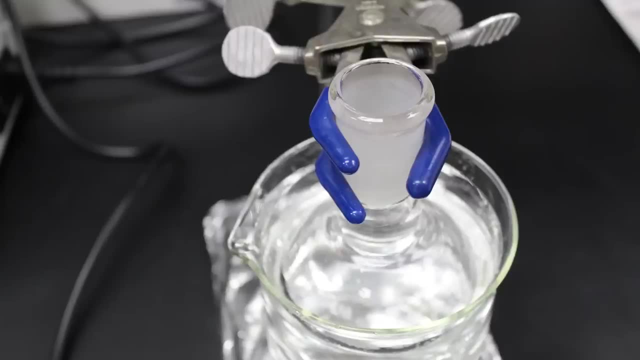 when possible. Clamps themselves are very adjustable, with several screws, And there are a few different styles in terms of precisely how they grip the glassware. Familiarize yourself with these, as we should know what kind of clamp will work best with a particular piece of glassware. 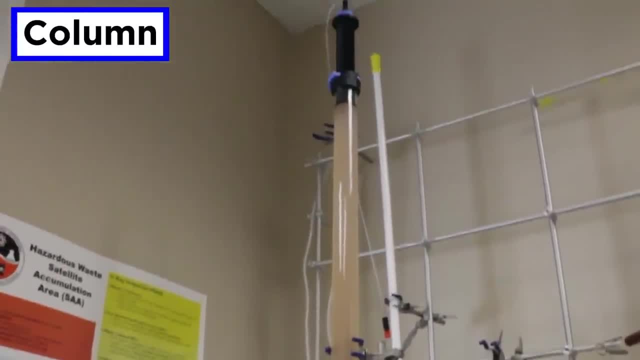 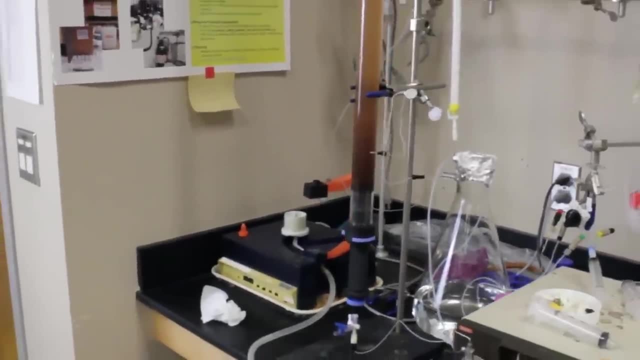 Now here, this lovely instrument is a column. We use these when performing column chromatography. They are essentially big, long glass tubes with a valve at the bottom, Some have a ground glass joint at the top and some have solvent reservoirs. Some have a ground glass joint at the top and some have solvent reservoirs. 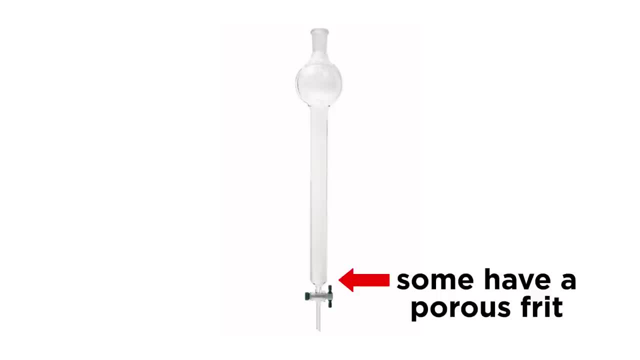 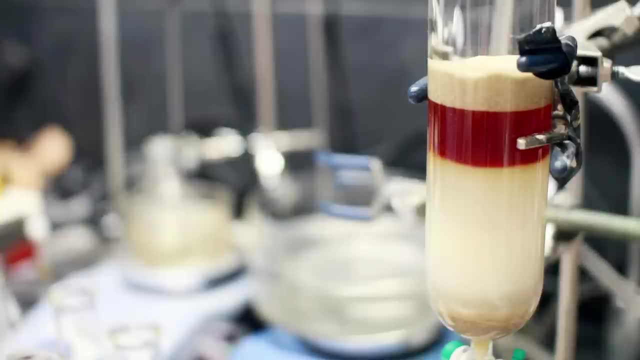 Some have a ground glass joint at the top and some have solvent reservoirs. Some have a frit at the bottom, which is a porous material, and some don't. We will learn how to assemble and use one of these in a later tutorial, but for now, 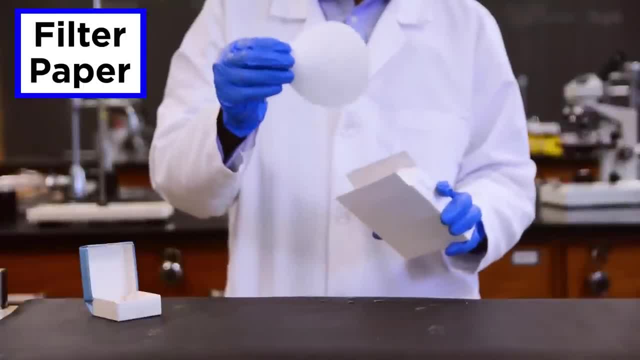 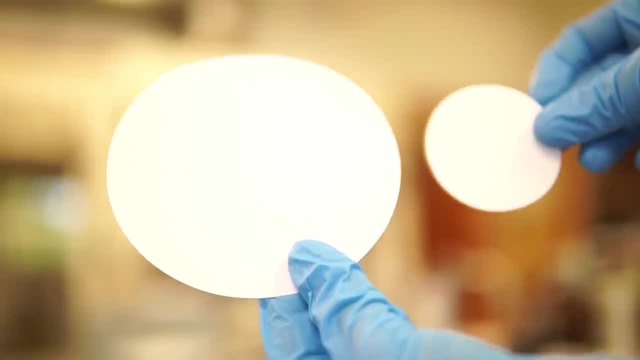 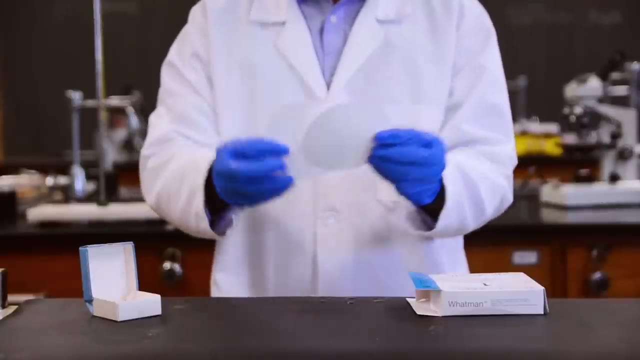 we know what they look like. Now getting to some of the smaller accoutrements. this is filter paper. Filter paper comes in various sizes and gratings depending on the size of the particles you are filtering. Generally speaking, a finer grating will filter a solution more slowly. 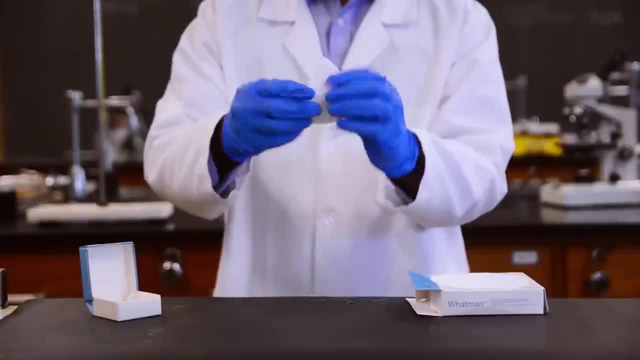 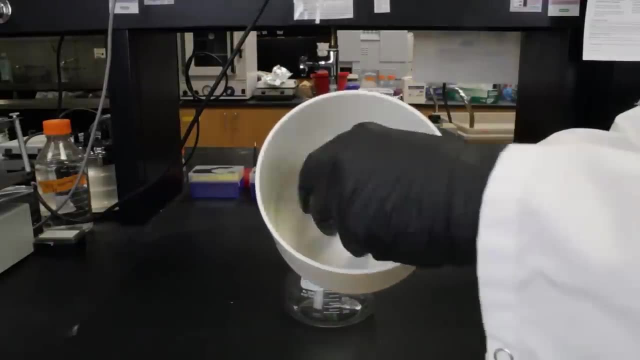 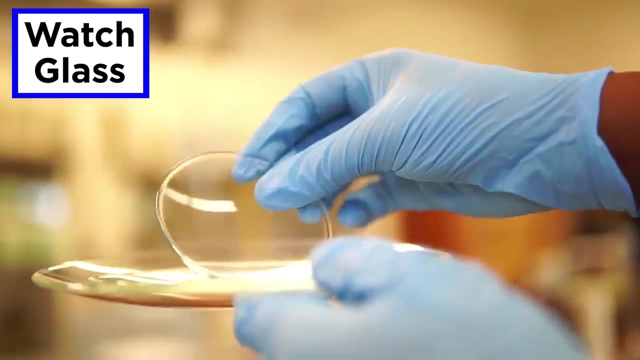 Filter paper will be used for the Buchner filtration setup, but can also be used for gravity filtrations, which we will perform later in the series. Filter paper can also be used to passively dry solids, as they tend to absorb liquids. Now, this is a watch glass. 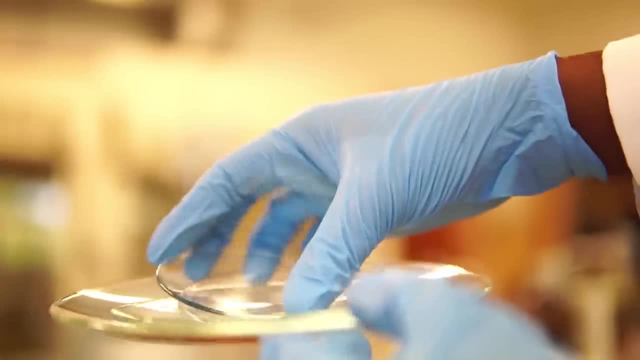 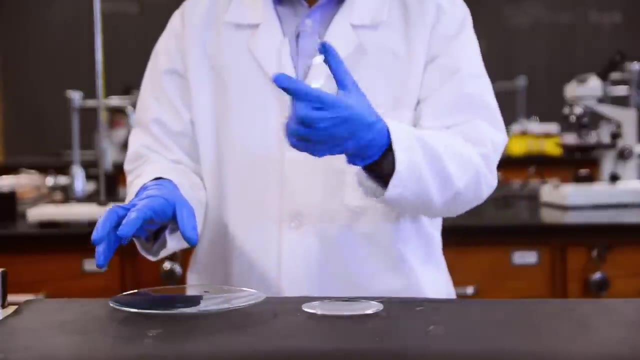 A watch glass is just a simple piece of glassware that can be used to hold and weigh an amount of solid. They wobble a bit, so be gentle with them. Similarly, this is a watch glass. This is a watch glass. This is an evaporating dish. 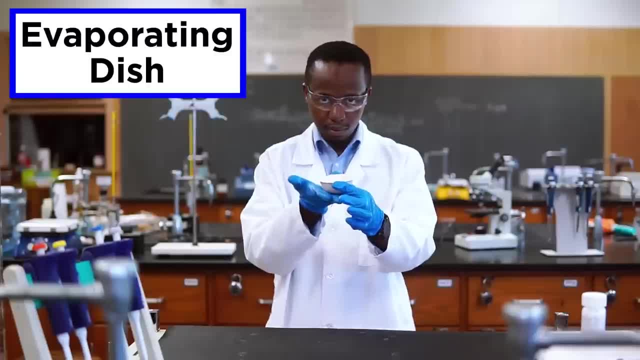 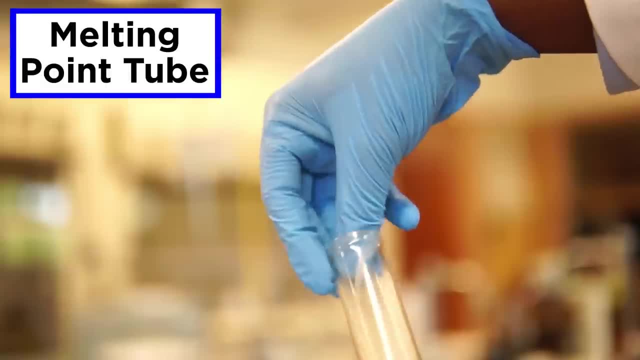 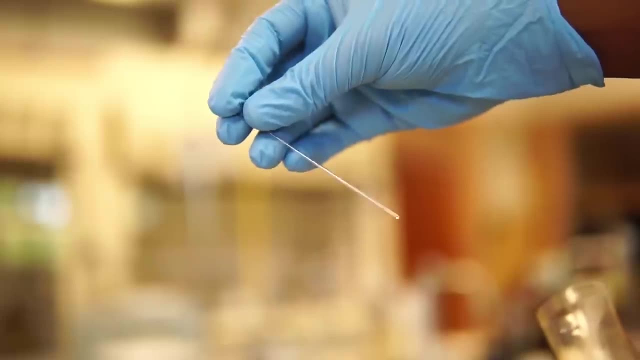 Sometimes you may need to let a wet, solid sit and dry. We can use an evaporating dish for this. They are typically ceramic and have high edges. Now this little thing is a melting point tube. When performing melting point determination, you need a melting point tube. 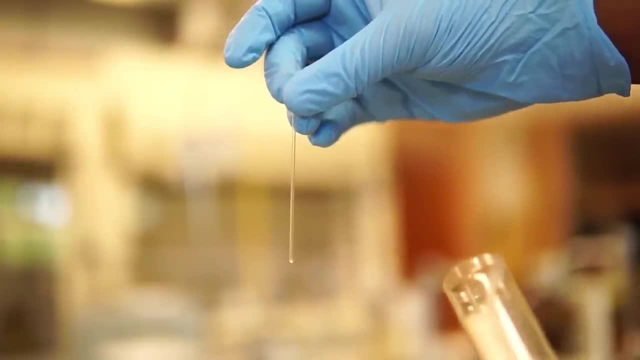 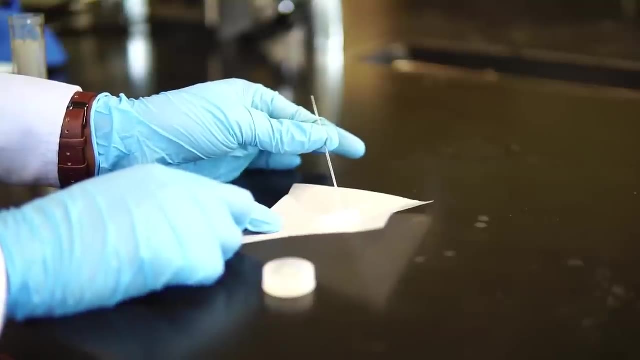 These look like little capillaries, but they are in fact sealed at one end. They are very thin and small, so make sure you have an area where you can safely place them. The solid is added to the open end and the tube can be placed in any melting point apparatus. 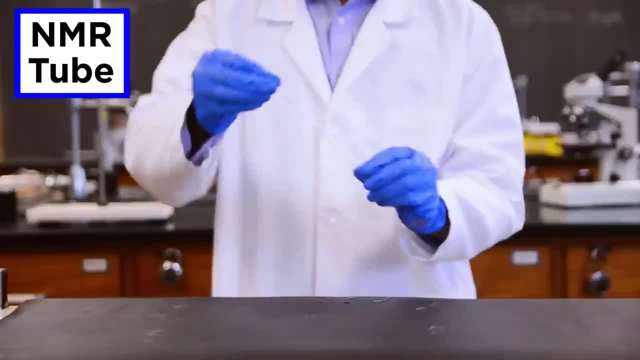 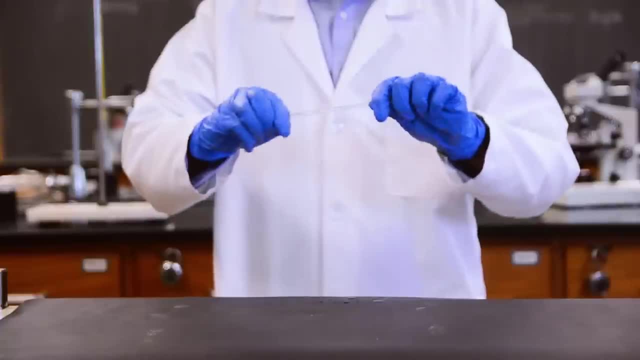 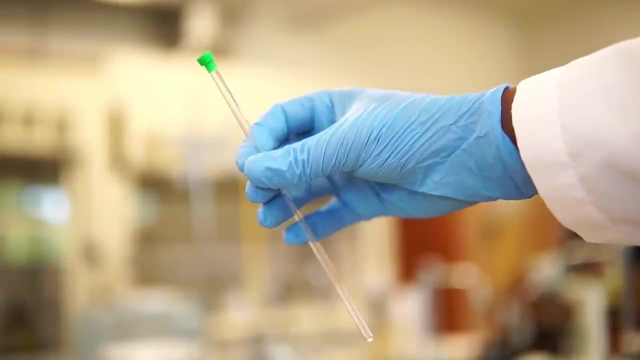 when measuring the melting point of a compound. In the same vein, here is an NMR tube and cap. When you need to obtain an NMR spectrum, this is the tube we will use and here is the cap we use. Simply make a rather concentrated solution of the compound you'd like to run. add it. 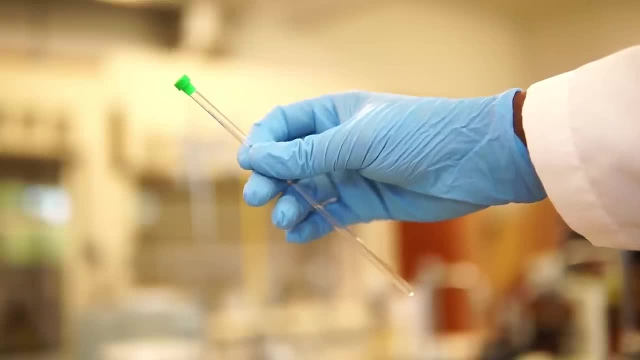 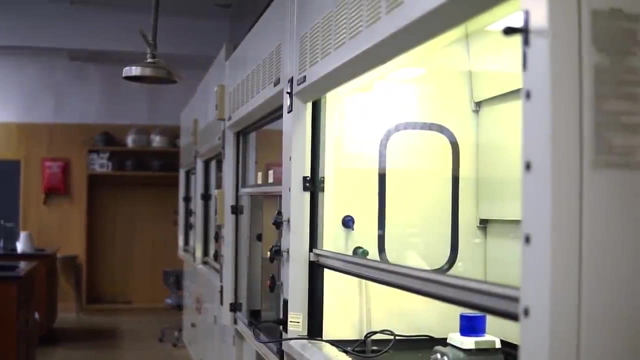 to the tube with a pipette and then cap it. This is now ready for the spectrometer. Now let's head over to the fume hood. We will tend to run reactions in here, so many instruments will live inside the hood. 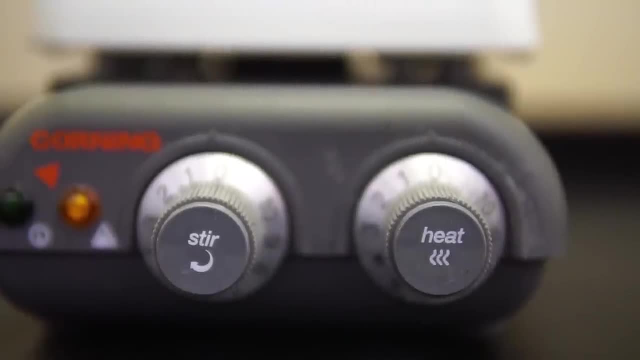 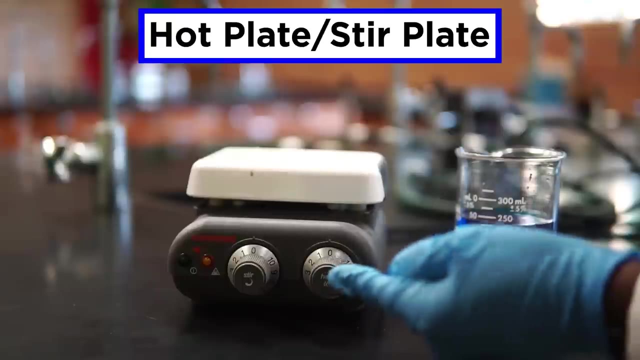 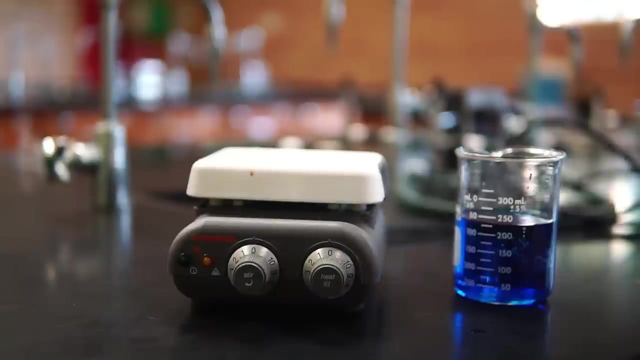 This is a combination hotplate and magnetic stirrer. As one would guess, this piece of equipment can both heat and stir your reaction. One dial will control the heat and the other will control the rotational speed of the magnetic stir bar. The heating may need to be calibrated, as the dial may not be totally accurate. 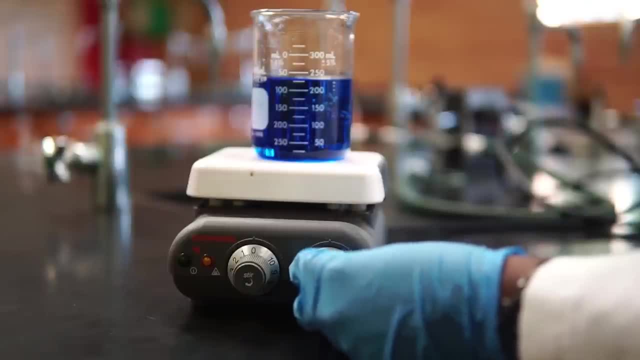 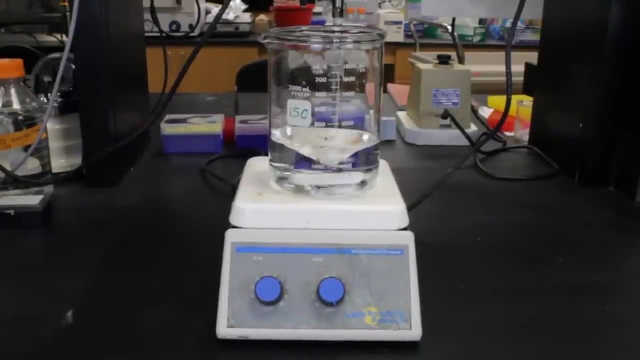 Some have a plug for an external thermometer to be used, so keep an eye out for that. As for the stirrer, a small Teflon stir bar can be placed in the solution and the contents of the reaction flask will be mixed like so. 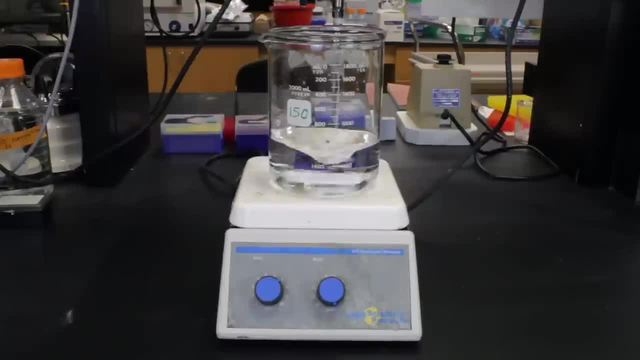 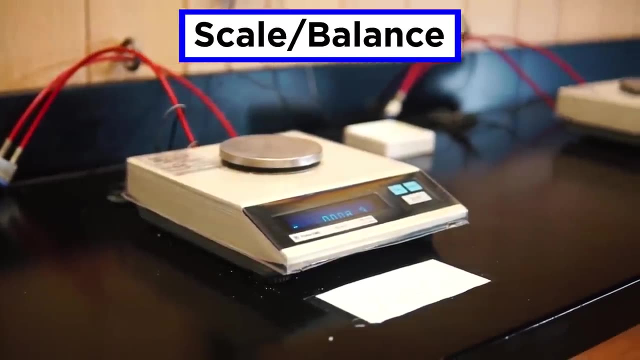 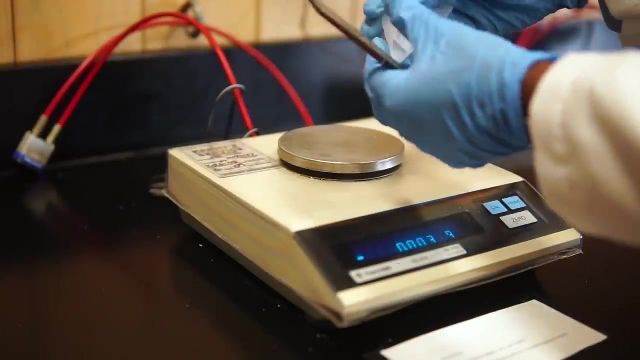 The stirring can get quite aggressive, so be sure to clamp up the vessel to stop it from possibly falling over. Another indispensable piece of equipment is the scale, or balance. Scales are used to weigh the mass of solids accurately. Be sure to tear the scale with any vessel you are weighing.